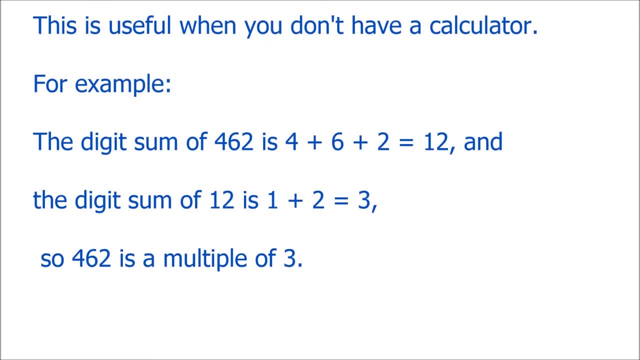 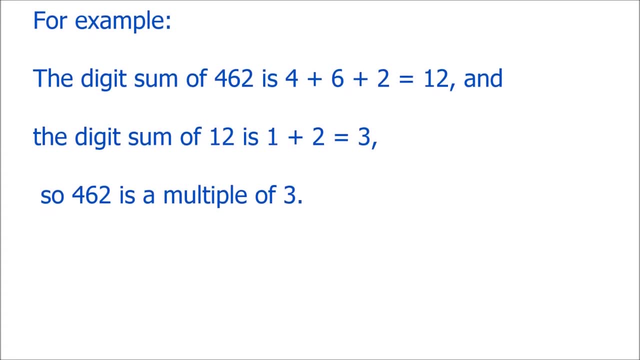 So we add 4 and 6 and 2, which gives us 12.. And then either we can say: well, 12 is a multiple of 3,, so we know that 462 is a multiple of 3.. Or we can apply the digit sum rule again to 12.. 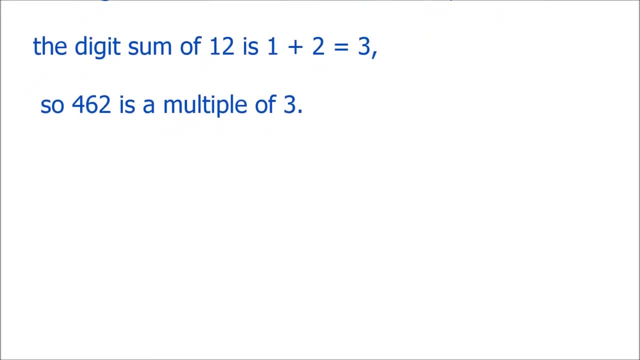 So we add together the digits in 12,, the 1 and the 2, and we get 3.. So we know that 462 is a multiple of 3.. You may like to try this method out on the bigger numbers in Pascal's triangle. 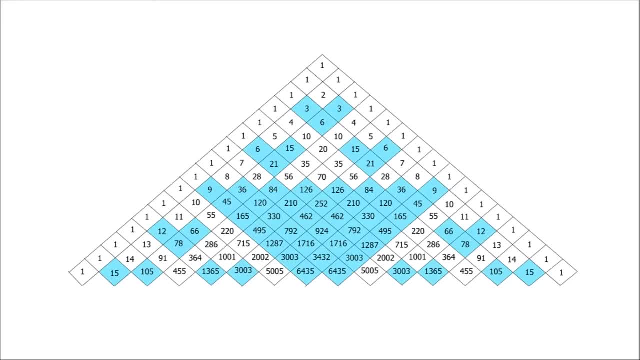 Whichever method you use, this is the pattern you should get in Pascal's triangle when you shade in the multiples of 3.. You may like to compare this with the pattern you got when shading in the even numbers. Other things to look at are what would happen in the next row of this triangle here. 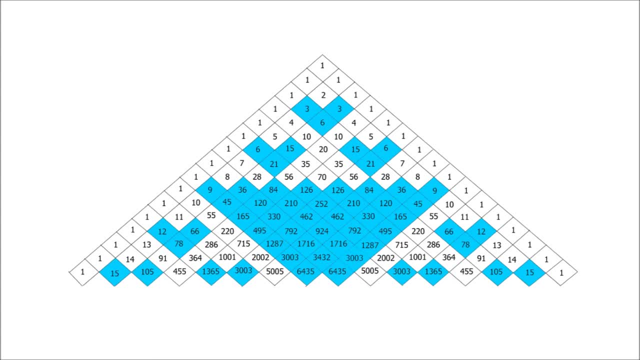 Where would you be shading in? One way to think about this would be to think about: if you're adding together two numbers which are multiples of 3, would the answer also be a multiple of 3?? And if you're adding together one number which is a multiple of 3 and one which isn't? 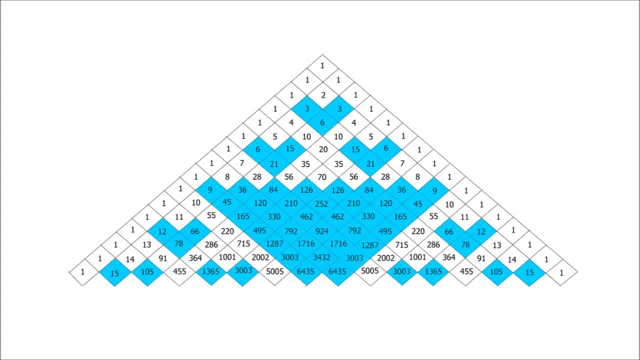 would the answer be a multiple of 3?? That will help you predict what's going to happen next. Something else to think about is to look at which rows have no shading in them. So look at the triangle we've got here. Think about which rows don't have any shading, in which rows have no multiples of 3 in them. 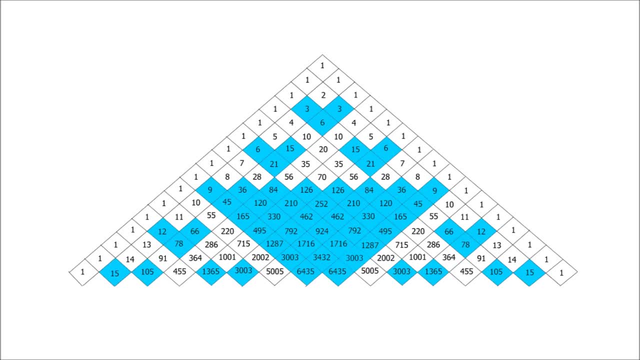 And can you work out which row will be the next row that has no multiples of 3?? Once you have finished looking at multiples of 3 in Pascal's triangle and you've looked at multiples of 2 in Pascal's triangle, then you might like to look at Pascal's triangle again. 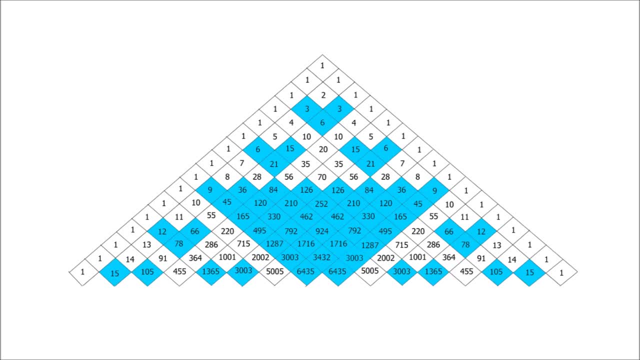 but this time shading in multiples of 6..